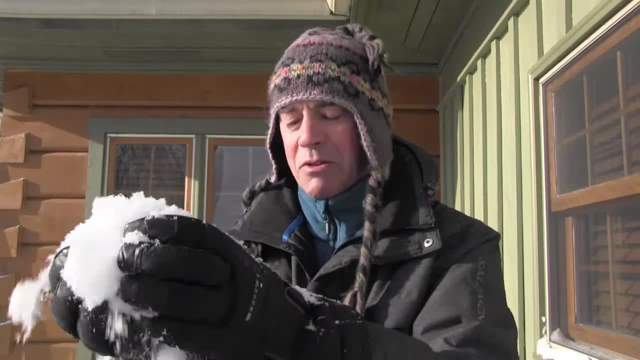 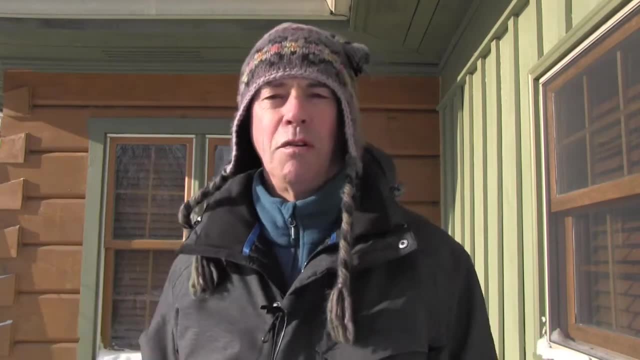 the snow that we have here right now. this snow here is actually powder, so it's not a brilliant example for what I want to talk about, but if you think of the shape of a snowflake, if you think of the sort of classic shape of a snowflake, every little bit of the snowflake, every individual lobe. 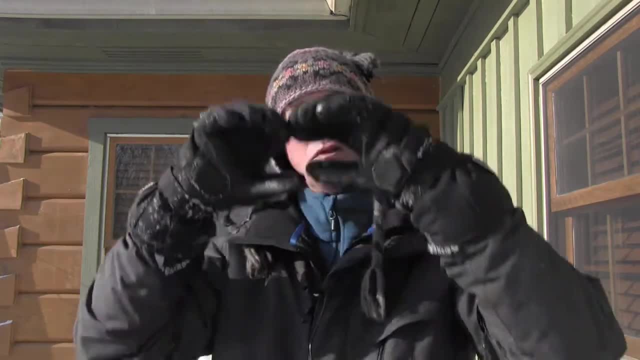 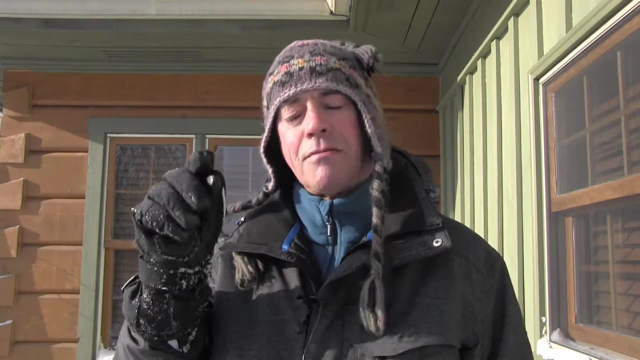 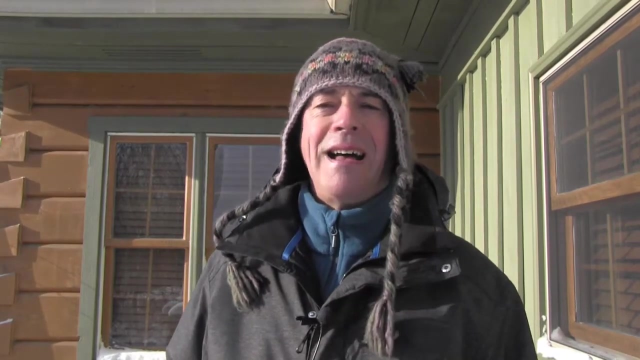 of the snowflake has the same shape and structure as the overall snowflake. So actually a snowflake represents a fractal, or the little lobe of the snowflake represents a fractal of the bigger snowflake. and the reason this is interesting is that it was one of the first profound moments I had. 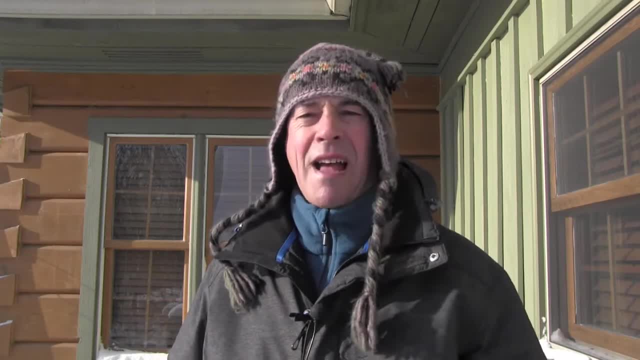 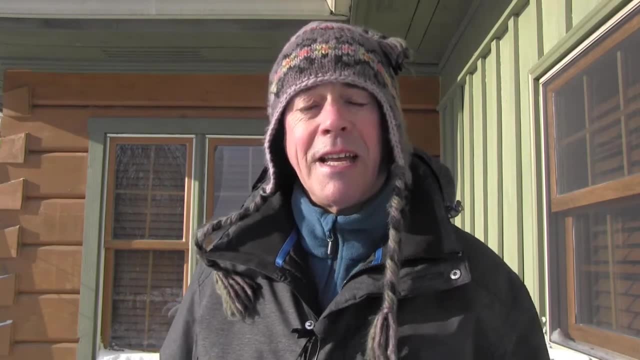 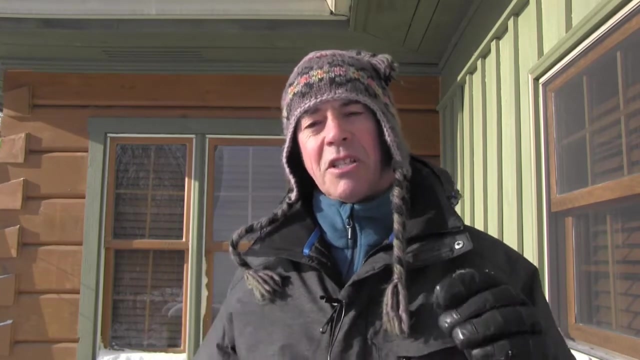 when I was training to be a therapist, I was wondering how therapy, how psychotherapy, actually helped people. and my mentor, Patricia Clarkson, said: well, you know, therapy is like a fractal of your whole life. If you change something in therapy because it's a fractal, because it has 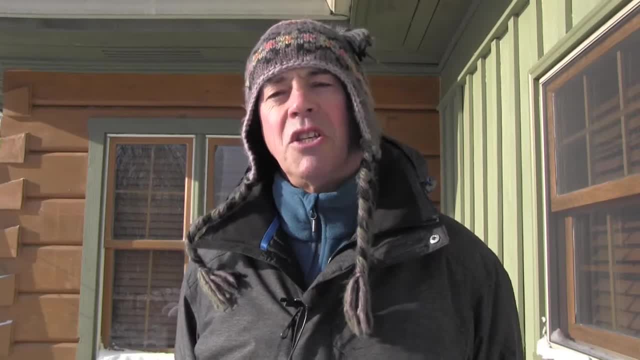 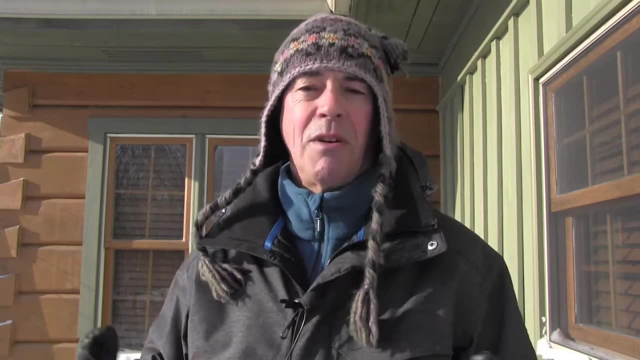 a self-similarity. if you change something in therapy, then it also has to change the relationship of that thing to the whole world And interestingly that feeds into systemic therapy as well. If you think about it, a family is a system, and if you change one element of a system then everything else has to change. 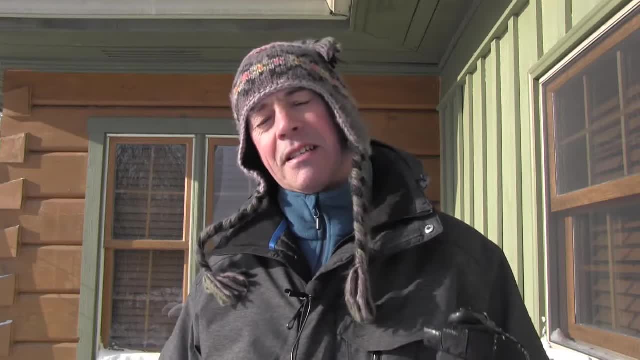 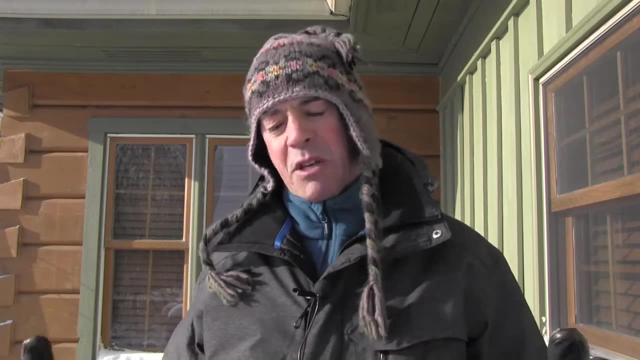 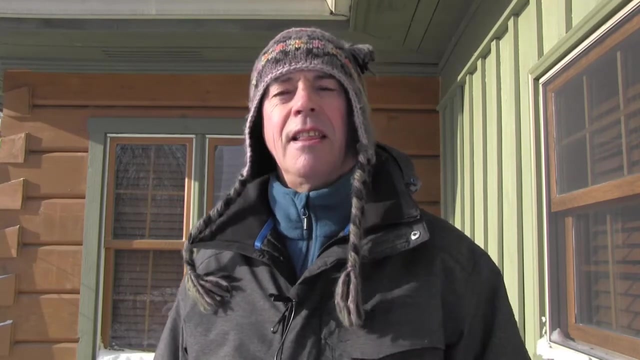 to accommodate it. So that got me thinking about how therapy works and how you know therapists can help people to change their lives, Because of course, changing a life is a really difficult thing to do. but changing a little thing is not that hard to do, And when you change a little thing, 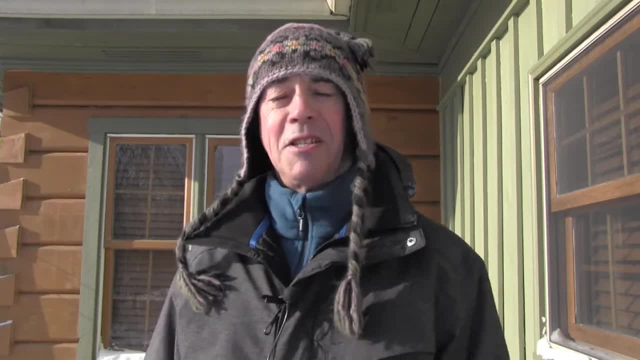 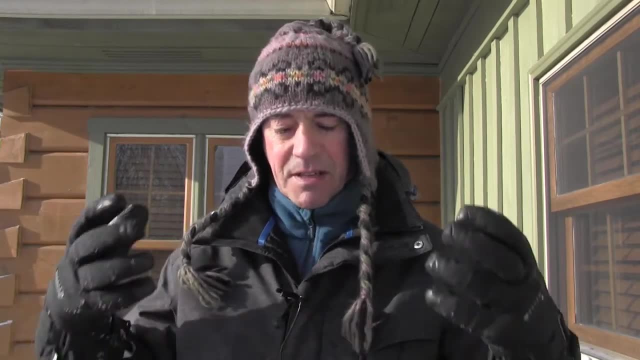 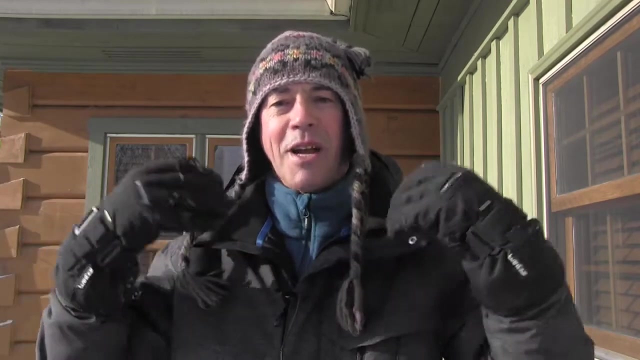 everything else also has to change. So I devised this motto which I still use and I find it quite interesting. I say to people- you know you may have heard this in my other films I like to use the human computer analogy, so you know, like where computers in a sense, or human computers, hardware, software, 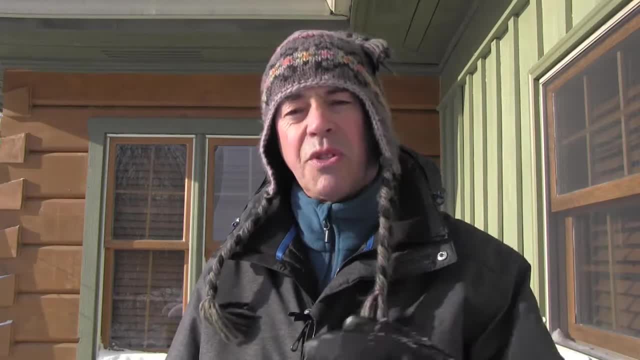 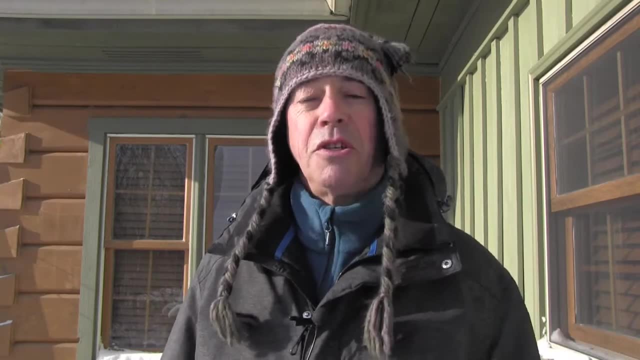 and the programs that we run in here are really beliefs. they're thoughts, they're expectations, but really, let's just say, a belief is a program. If you're running a program on your computer, you expect to get an outcome, because that's, if you run a program and nothing happens, you'd feel cheated. 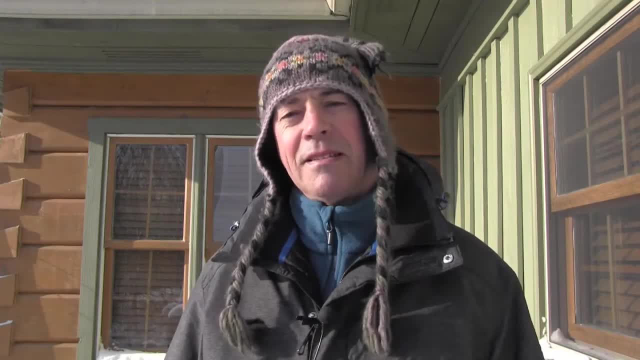 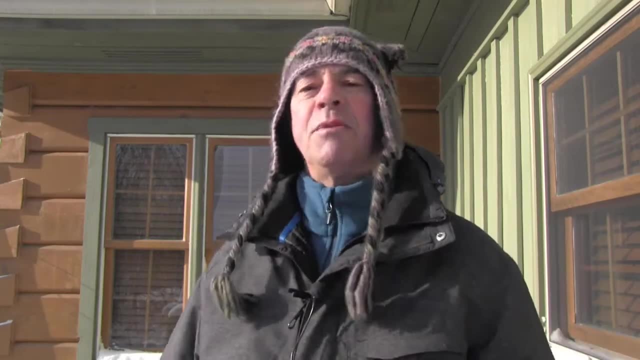 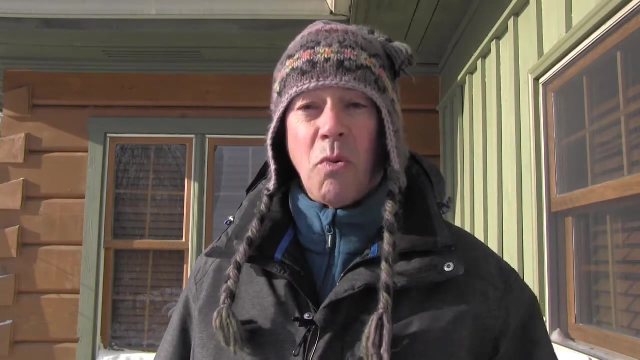 So running a means that you're going to get an outcome. now, when i work with my clients, you know we spend a lot of time figuring out what the programs are in here that are giving the outcomes that they don't want, and i often ask this question: what programs are you still running or what solutions are you still? 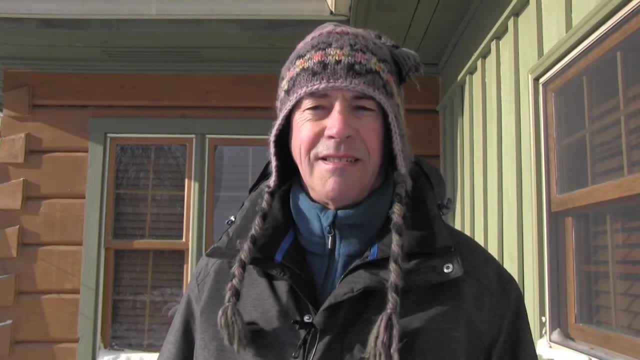 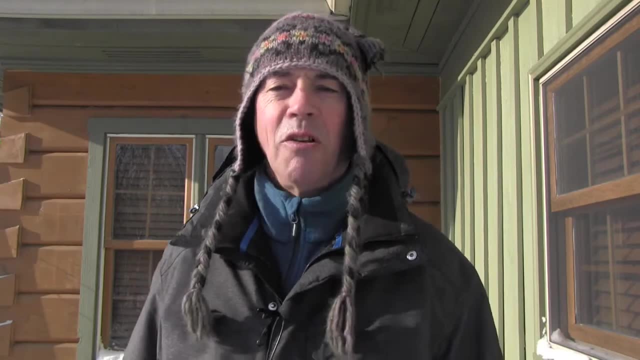 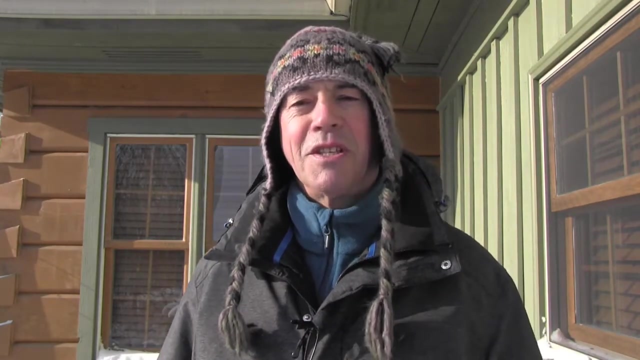 running in here to problems that no longer exist. so in a sense, a program or a solution got running to solve a problem, but the problem's long since solved and no one's told the program to stop running. i was talking to a client a while ago and i was using this idea of what solution is still. 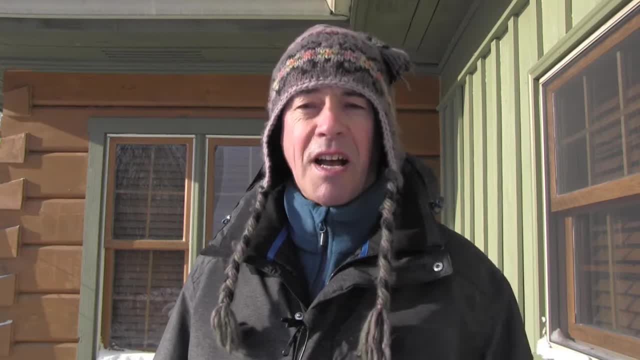 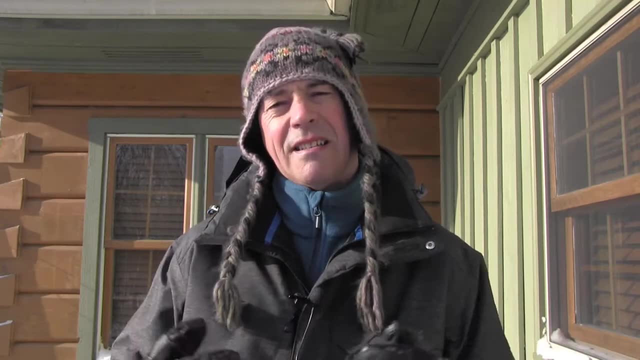 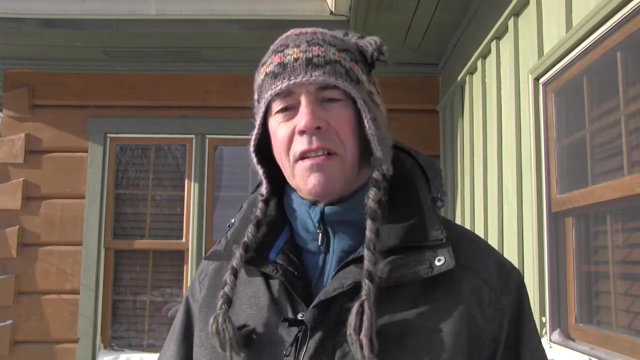 running to a problem that no longer exists. this person's retired and she said i always felt in my work that i wasn't respected or clever enough or that i'd always be sort of looked at as being somewhat inferior, and so that was how she felt. her solution was to have a lot of books, she said. i always felt if i had a lot of books in my house, 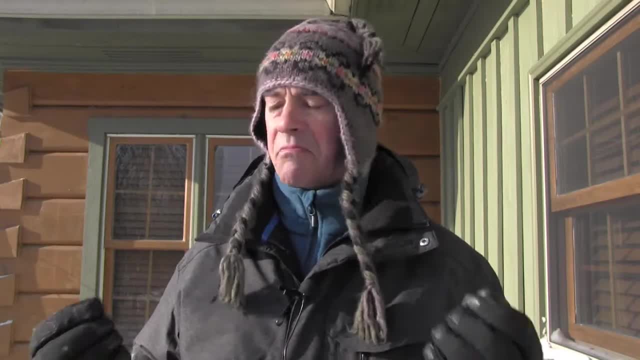 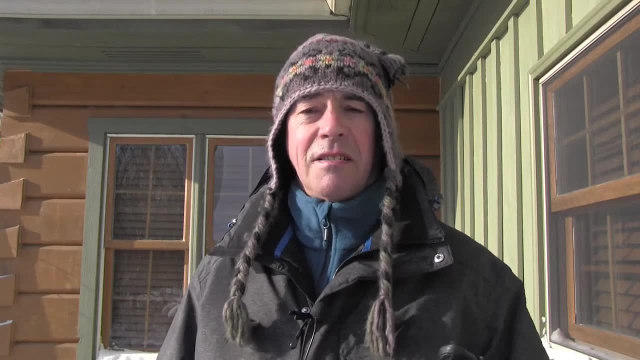 then i'd be taken seriously and i'd be, you know, i'd be respected for for being knowledgeable and academic. but of course, now that you know she's retired, there's no one really to judge whether she's you know, academic or or good enough to do the job, because she's, you know, retired doesn't. 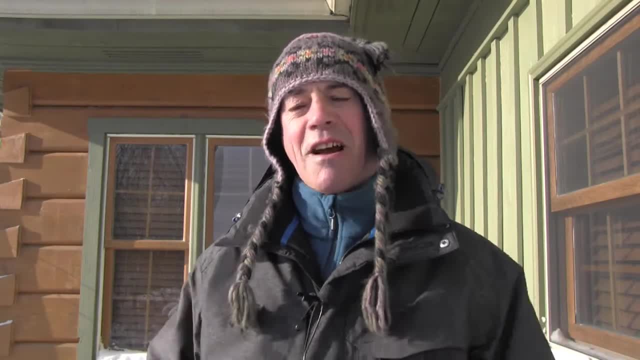 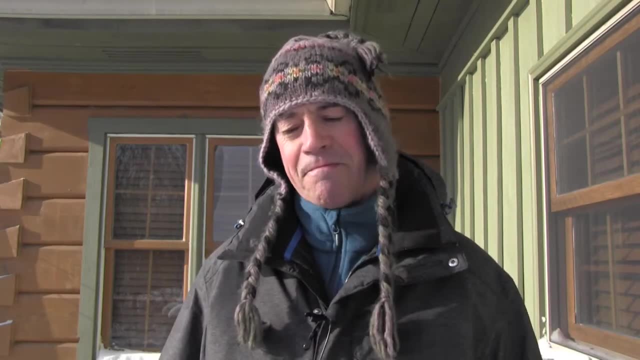 need to do the job. the problem is that the house is full of books. and now the house is so full of books that actually it's necessary just to declutter the house to get rid of some stuff, but still likes to buy books. now you know, buying books is a nice thing. 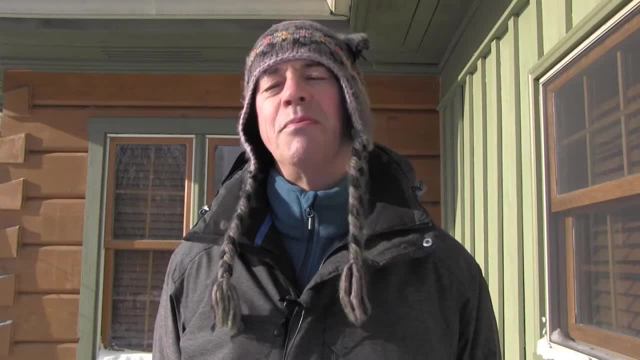 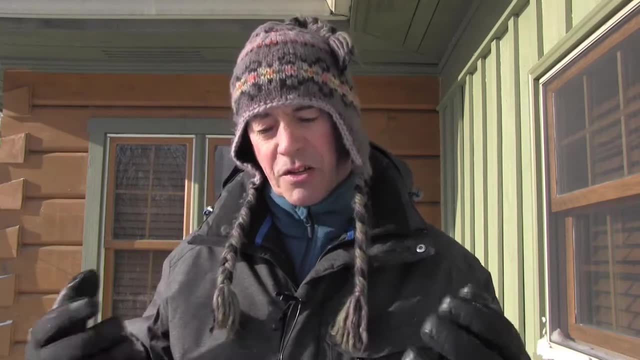 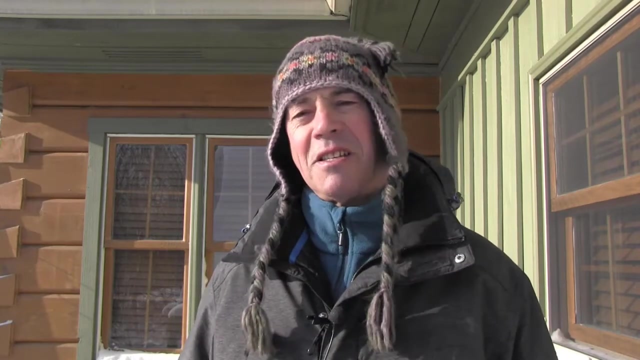 but in principle, buying books and having books and keeping books is the solution to the problem of feeling inferior or not good enough or not not going to be respected by colleagues. so buying books is a pro, is a solution to a problem that no longer exists. so that's quite an interesting 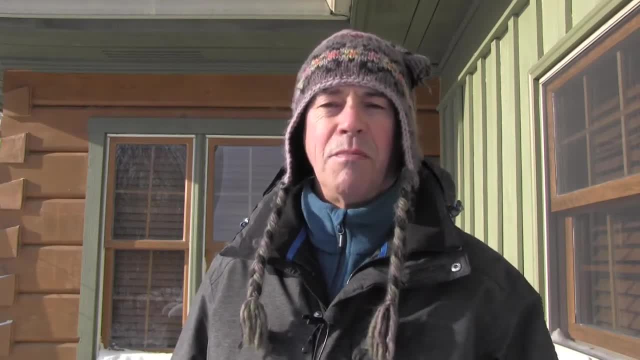 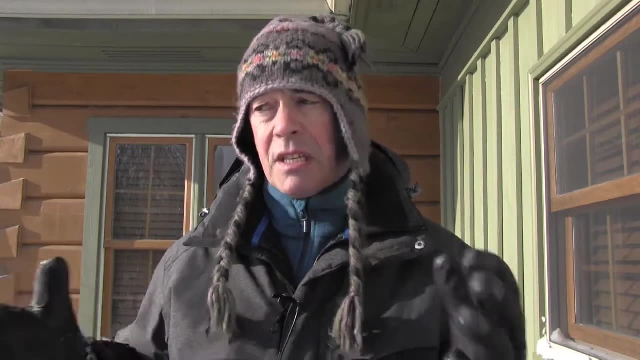 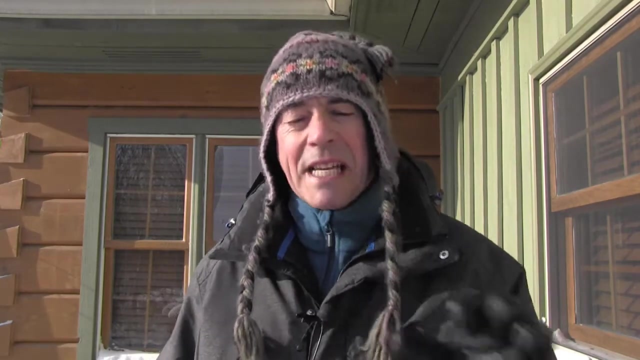 example. another interesting example, i think, is from the world of feeling anxious and feeling fearful. often, things that happen to us in life are very frightening. you know, we get a tremendous shock. it's like a, like a road traffic accident, for instance, or any kind of experience where you feel. 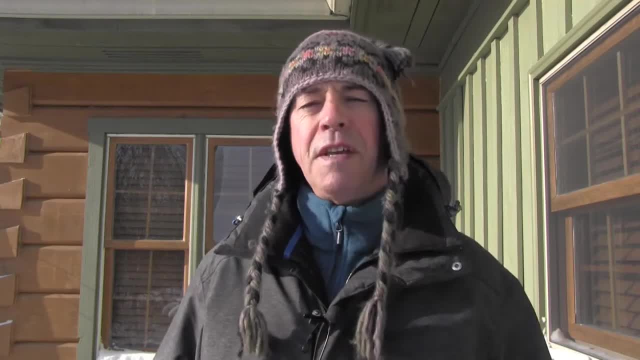 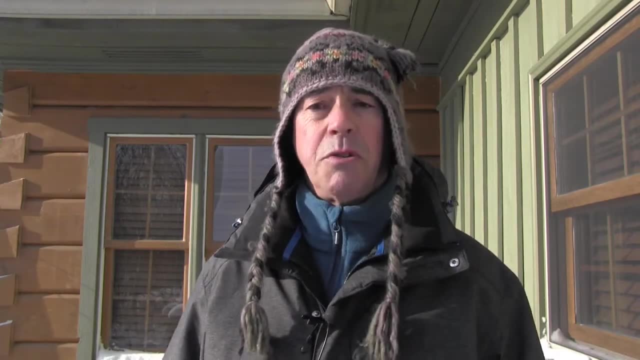 you might die, or really any kind of panic experience where you feel that you know you're going to lose control of yourself. that's very frightening, it's very difficult to tolerate, and so what we do is we try to manage it as best we can. now. you wouldn't necessarily know why you. 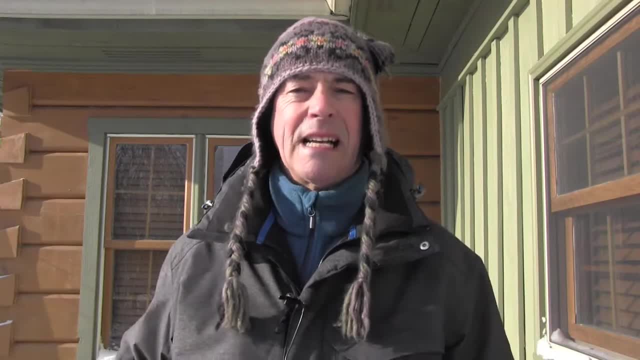 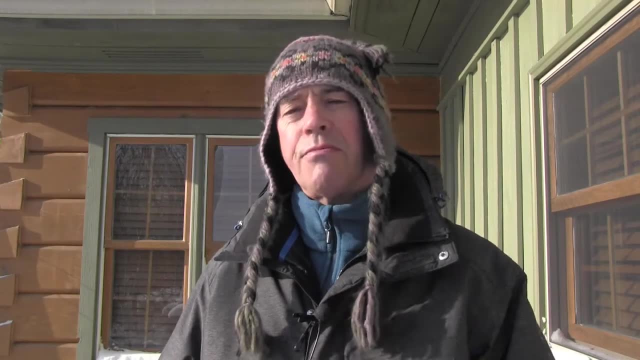 had this. if it was an accident, of course you understand, but if it's just like a panic attack out of the blue, you wouldn't necessarily know why you had that experience. so you have to manage it right. you've got to create a solution to manage that problem well. a lot of times it's avoiding. 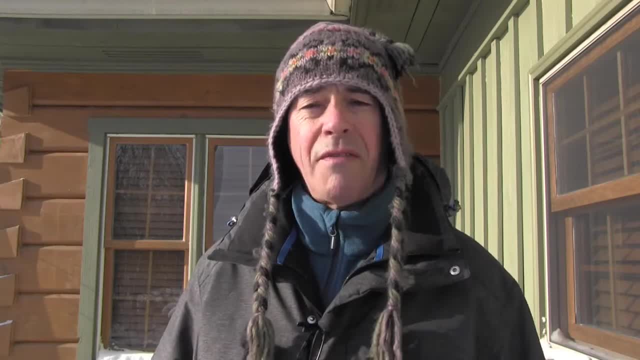 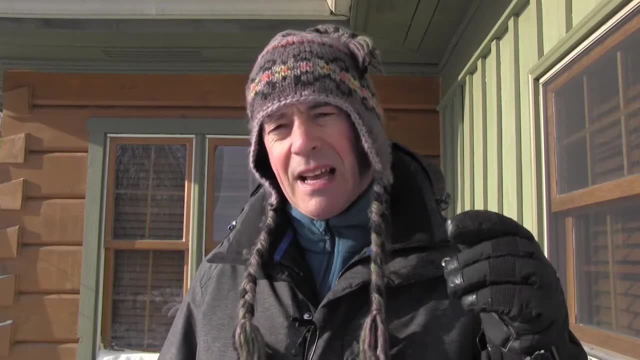 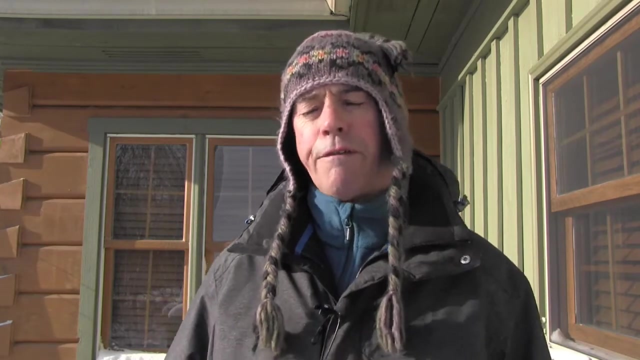 things. you know. if you have a panic attack when you're driving, you avoid driving on the motorway, for instance, or or roads where it's hard to get off, in case you lose control of yourself. so a solution is sometimes it's okay and sometimes it's not okay, but we tend to run solutions far longer. 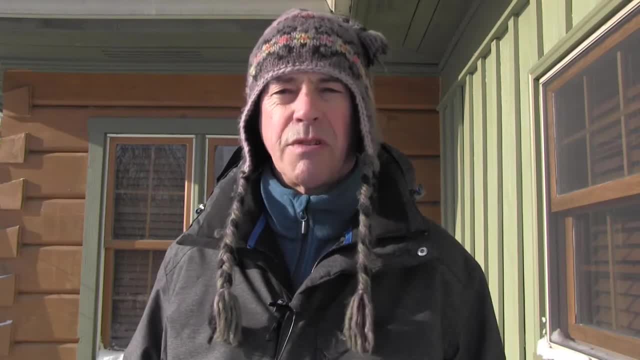 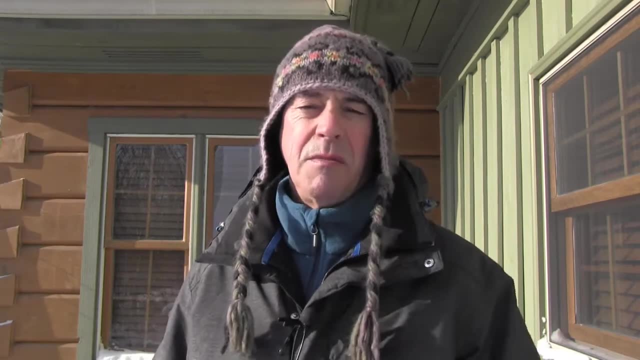 than we need to, because the problem no longer exists. so once you understand the panic experience, for instance, and once you get a little bit practice with breathing and some grounding techniques and some of the cbt stuff, well you know, the problem of panic really goes away. it's very hard to have. 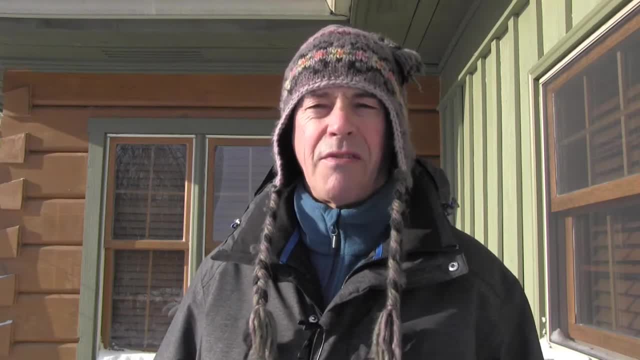 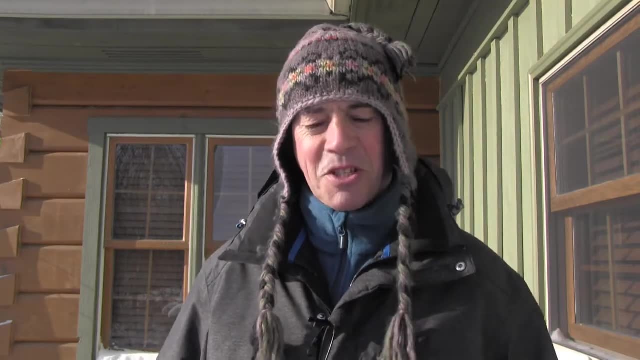 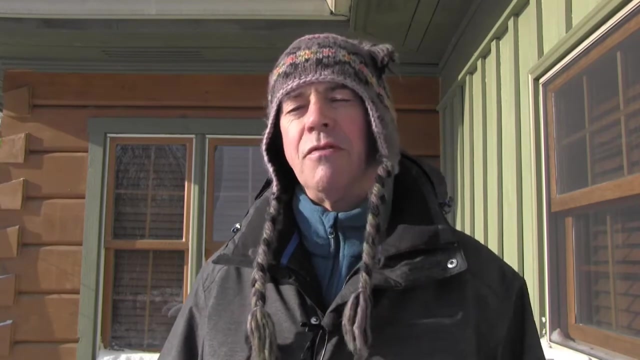 a panic attack. once you start really working on not having a panic attack, but avoiding the things that you started to avoid, that's much harder to overcome because you're still running the solution to a problem that no longer exists. so if you want to change some element of your life, how about this? find the smallest thing that you can recognize. 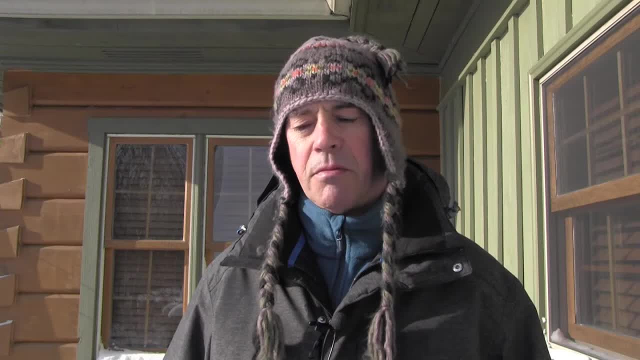 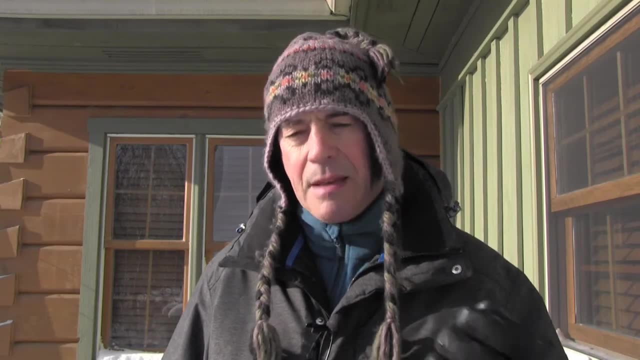 as being the thing that you want to change and ask yourself this problem: what solution am i still running to this problem? what solution am i keeping in play? even though the problem that i'm experiencing might not exist in the? i think it does, if you can find a really small. 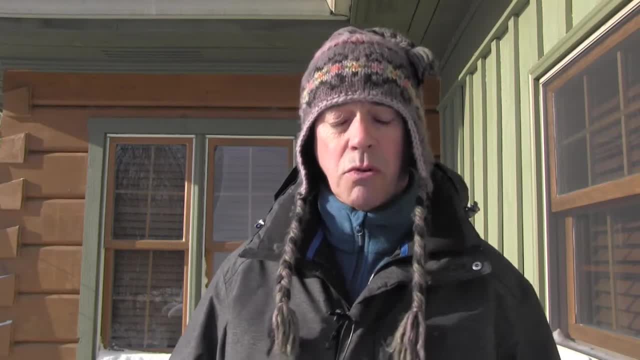 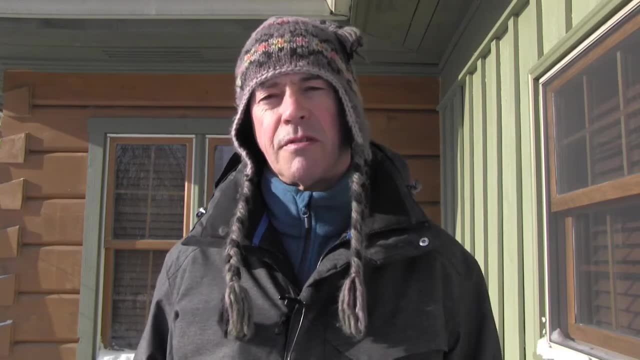 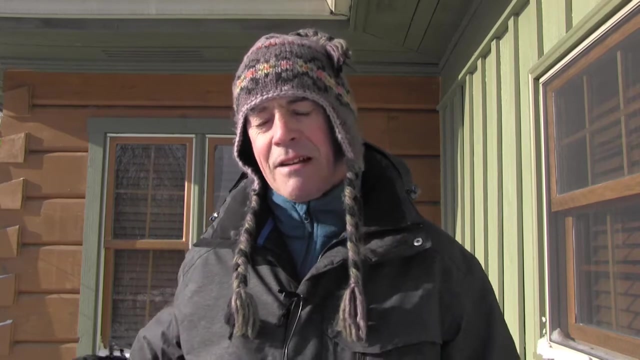 thing and you can change it. everything else has to change because of course we're a system and in a system everything has to run smoothly, otherwise the system doesn't run. so what solutions are you still running for problems that no longer exist? have a think about it. it sounds like a kind of 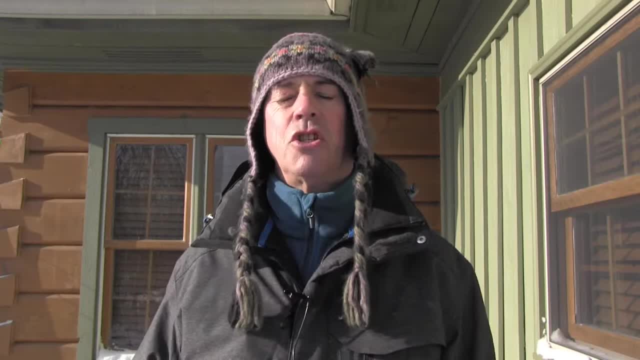 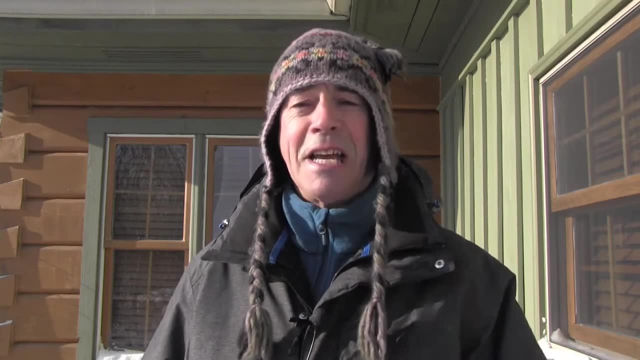 a mysterious kind of statement, but actually you know it's interesting and it has the potential to help you just to focus on some stuff that, in fact, is completely redundant and you can get rid of it in your life. see how you get on, let me know how it, how it sits with you, and let me know how you get.